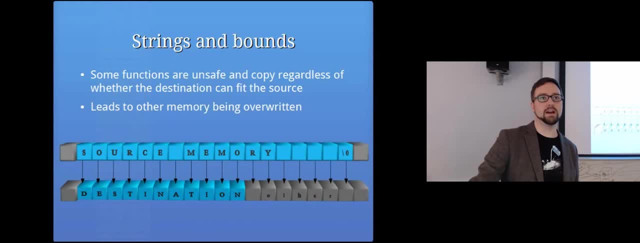 Java, if you try and copy too much into into an array, for example, you try and write into an extra element that isn't there, it'll just raise an exception and just say: no, you can't do that, that's a problem, basically, whereas in C, yeah, fine. 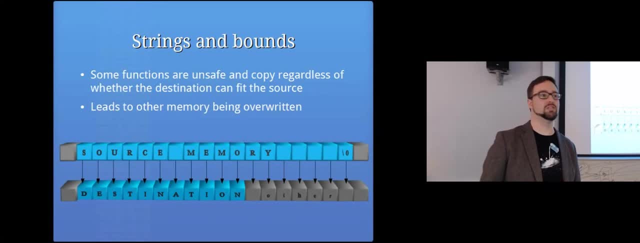 If you've got an array that's 15 characters long and you go, I want to write into the 100th character in this array. fine, just ends up some random place in memory. it's overriding something. Yes, it's not specific to an operating system. 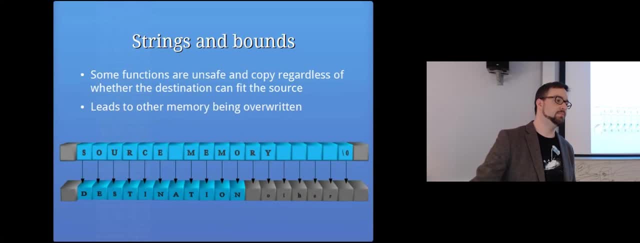 it's just the programming language isn't particular with those sorts of things. so yeah, it'll happily let you do things that just make no sense. but that's because that's your job as a programmer and to know what you're trying to do and the programming language just doesn't make sense. 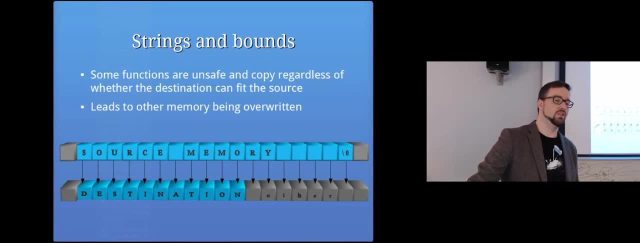 It does stuff basically, whereas as time's gone on, programming languages have tended to be a bit more protective and make sure that what you're asking, you know, makes some sense. so it is better if you're writing a piece of software if performance isn't important, if you choose a language like Java or C sharp. 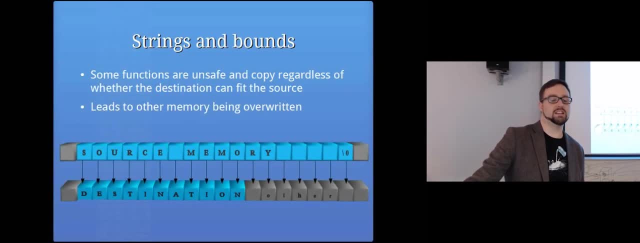 if you're so inclined, is. it protects against these kinds of mistakes being made. it'll still allow other kinds of mistakes, which we're about to talk about, but this specific problem of buffer overflows becomes harder to do. so you see, in this example in the diagram, we've got some source memory and in C the end of a string is: 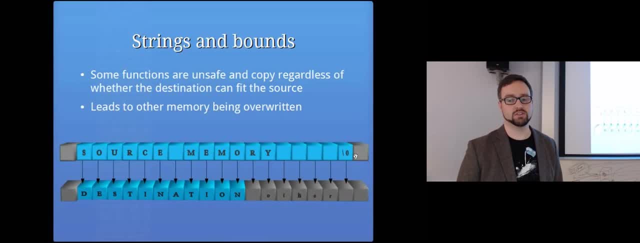 represented by the null character, which in C looks like a slash zero. so it's like a null character, and so everything up to that is considered to be the string, and if you try and copy it somewhere else, the it'll basically just happily copy all of that across, even though the 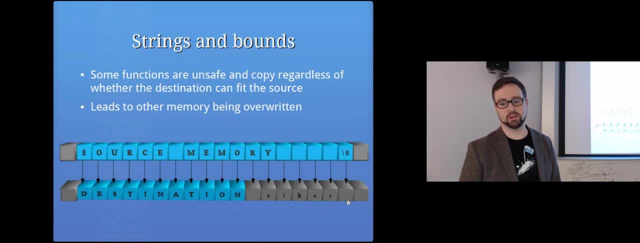 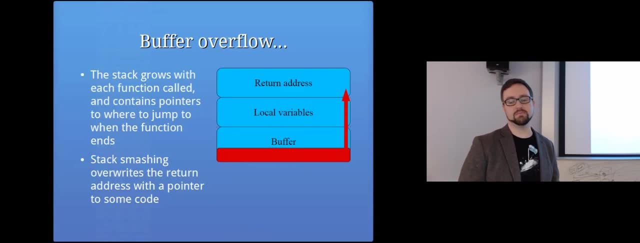 actual space that have been allocated to that variable is smaller. it has put the contents over the top of whatever was supposed to be there. so basically, a very simple example or description of buffer overflow is that every time your function, every time your code is running and a new function is called within your code, the stack kind of grows. 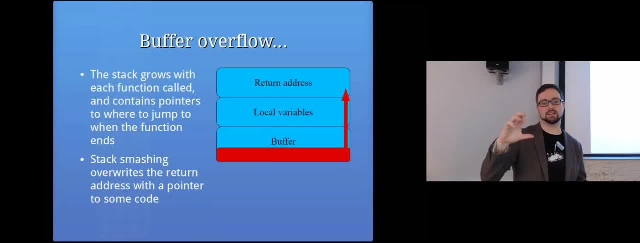 to have a new stack frame, so some space on the stack to represent this function. that's currently been called. but in order to remember where to get back to the code it came from, there's a return address there, so that normally points back to wherever the code was before we, you know, called. 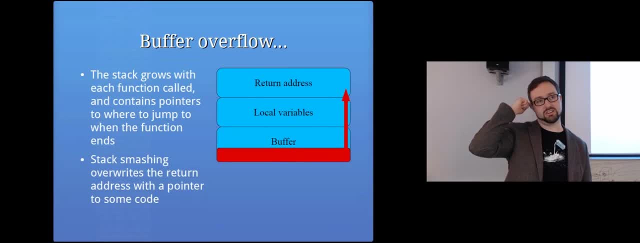 this function, but because of the way that it's structured, if you've got a buffer that's growing with stuff that you're copying over it, you can. you copy something into the buffer and you're not protecting the fact that you're only copying into some way that makes sense. you might end up overwriting the return address so that then instead 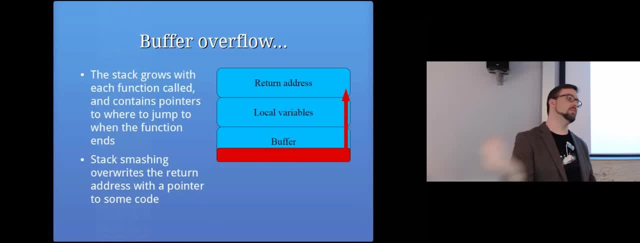 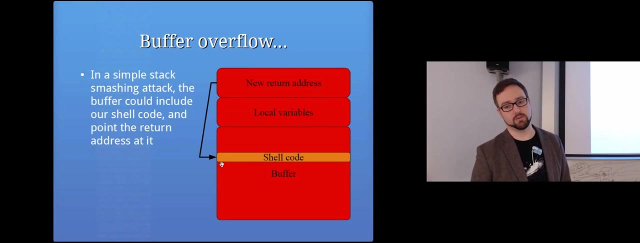 of just the code. when this function ends, instead of just jumping back to where it came from, it jumps wherever you want it to jump or wherever you've managed whatever address you put it into that spot on the stack. so in the very simplest example looks a bit like this, where we've got our variable and we write some, basically right. 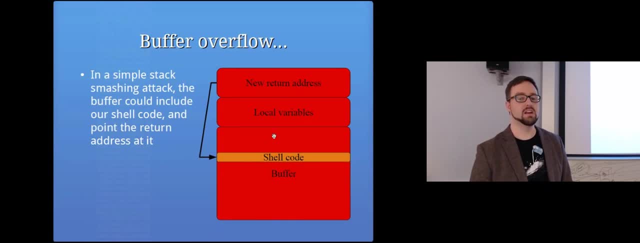 into this buffer that just is clobbering over everything else. we keep writing into it, keep writing stuff. we overwrite all the local variables and we end up overwriting the return address. and if we do things very cleverly, we might actually be able to point this return address at somewhere in. 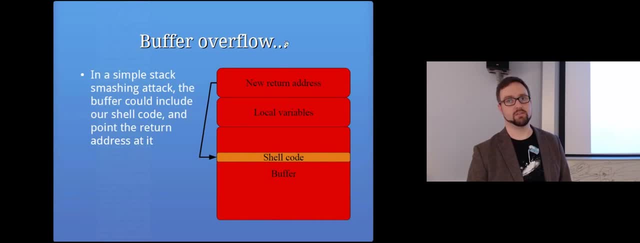 the middle of this buffer that we've just created. you know that we've just been overriding with stuff to control the input of all this stuff. this is all the stuff that we're entering into the program. we might actually include some shell code there, so some of the our own code, and then, when it hits, 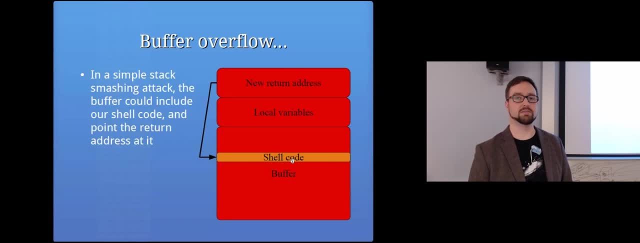 that return address jumps into our code. it's now running some code that we've written and put onto the buff, into the buffer, so the the program ends up executing our code instead of the correct code for that program. um, so I've just been in my office just now drawing this diagram because I think it'll help to clarify. 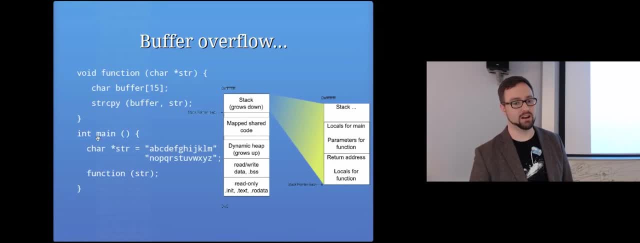 things. so, um, basically we've got our main function. so here's some C code: uh, in this case this demonstrates a nice little buffer overflow. so we've got a um, a character, uh, string, and, as I said before, in C there is no string, it's just an array of um characters. but this is 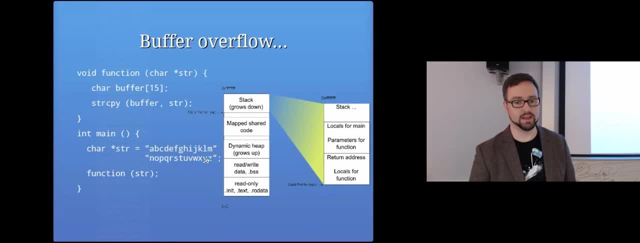 basically, um, creating this array of characters with the letters a to z in it, and then we're calling this function called function and passing in that string, and inside that function there's another string called buffer and it's got 15 characters: is the amount of space that's allocated. 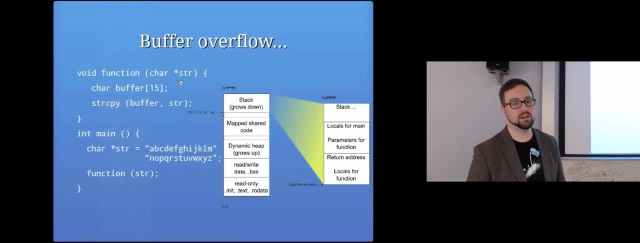 in memory and then we're just copying from the um, from the string, into the buffer. uh, this is going to fail, this is going to make weird things happen, because we're writing, obviously, this: uh, 26 letters in the alphabet into a space that only has 15 spots for it. so, as a result, it's going to 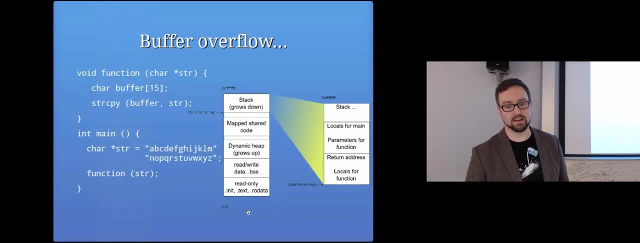 overwrite other stuff in the stack. so this is what the stack looks like, um, basically, um, it's a bit. it's. the confusing thing I guess about these diagrams is the stack grows down, so this is some memory. uh, that's for this program, that's running. and if we go down further down this way, that's towards zero, and if we go up that way, it's towards. 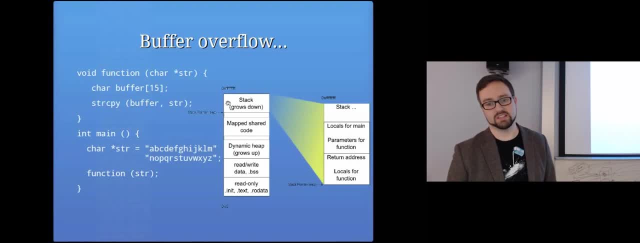 like the highest address space. um, the stack starts somewhere around, somewhere at the top, and as it grows it's actually getting to lower numbers, which, to be honest, always does my head in when I'm trying to explain things. and then you know, um, the there is also within memory for this. 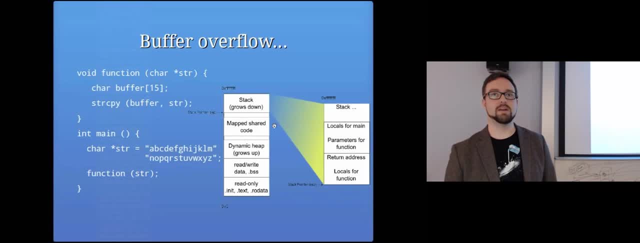 application. there could be some shared code like libraries and things that get mapped in um. there's a dynamic heap which grows up and that is um. basically, when a program wants extra space, so variables that are a bit bigger, for example, and it says: give me um one megabyte of uh space to use within this program, then it'll dynamically. 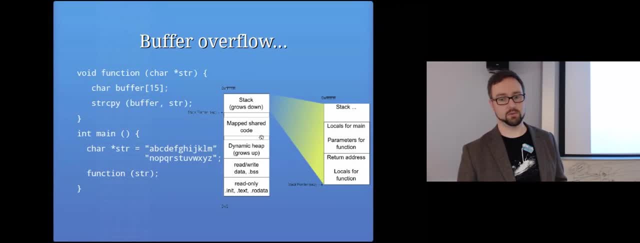 the operating system will dynamically allocate that space which becomes available in the heap. so that grows up, um, and then these things is basically mapped from the actual executable file itself. so stuff like the actual code of the executable gets mapped into these areas. so you know the thing that we're. 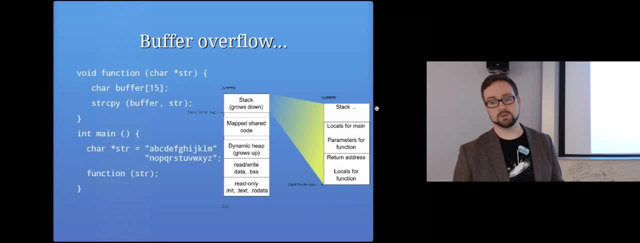 actually interested here is the stack, which is this part, the call stack. so if we basically expand this out, we can see that the stack has uh, amongst other things, we end up with the um. every time some new code runs, it gets some space on the stack. so here, when uh main runs, the 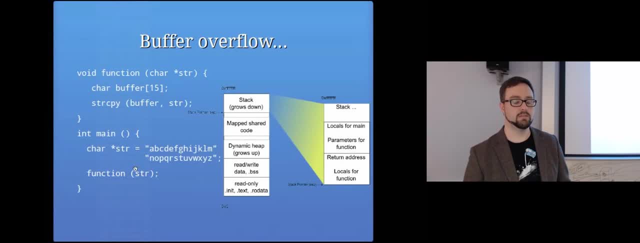 locals for main. so, like this variable, for example, would be sitting in the in num space here somewhere, um. and then we've got parameters for the function. so, for example, we're passing this in this pointer into the function, so that would be sitting in um on the stack. 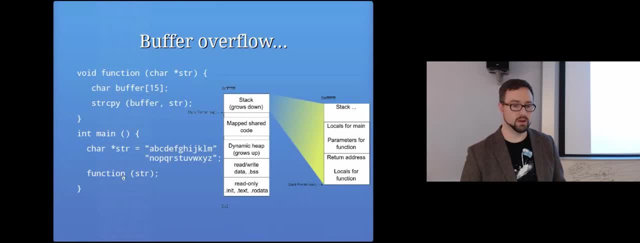 um. and then we've got um when we call, when we hit this part in the C code, and it starts executing the function here. at that point this extra bit of um stack, the stack grows to accommodate that. so then we get this little stack frame here which includes the: 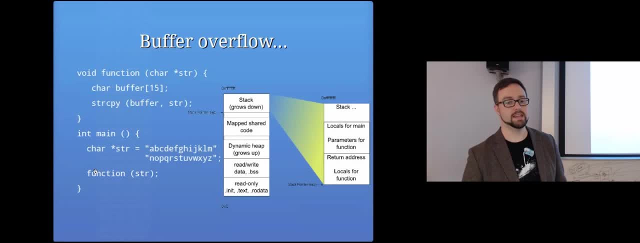 return address. so how to get back to our code: um here and uh, the locals, which is the buffer um. so when things go bad, we, instead of just overwriting the local buffer, we actually also end up overriding the return address, which means that we can change where that code jumps back to. 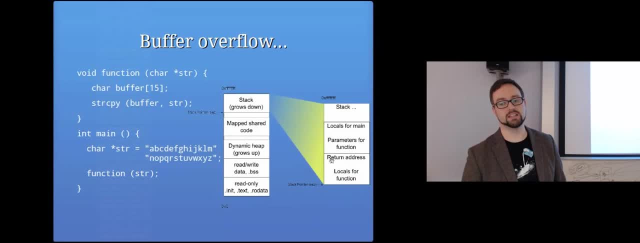 uh, because when the function ends it rereads that return address off the stack, back into register and that's where you have the normal. but this is a fairly commonס back to here. it'll jump wherever the hell we want it to, maybe down into some shared code somewhere. 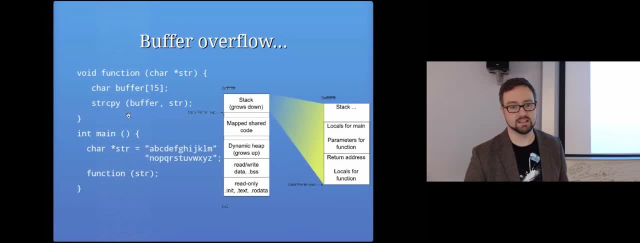 or somewhere else within the program, or just somewhere inside our buffer that we put, put a shellcode, some shellcode, yes, what memory is it actually using? is it using the memory of the processor, um, the ram, um, so we're talking. so we're talking about virtual address space. 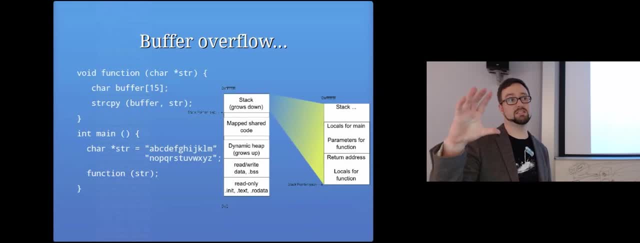 so each program gets some space and it it maps that into various places. so it might be that some of it is actually sitting somewhere else in the ram because, like these shared code mappings might not actually be sitting, might not end up sitting inside that piece of ram. but basically it's, it's abstract and the operating 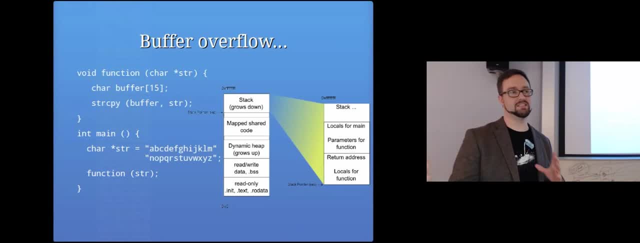 system does magical things to manage all this stuff and it does things like swapping things in and out of ram and onto cpus and and all that sort of stuff. but when we're talking about the, the address of memory here, we're talking about virtual addresses, so each program gets this range. 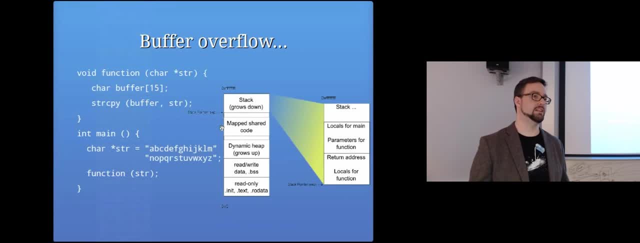 where it has memory which is basically sitting in ram. so can the same program architecture. it will. yeah, actually the code will end up being different on different architectures. so this c code will be the same, but when we use our compiler to create the executable, that will be separate programs. so if you wanted to compile a windows and a linux program from this same code, 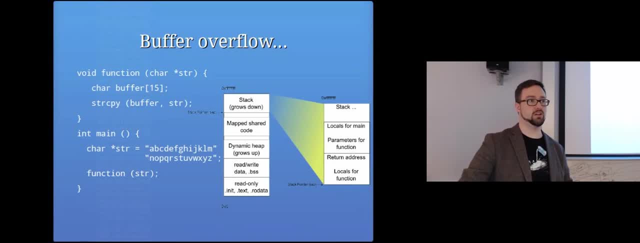 on Windows or Linux. but when you compile it it will generate separate program, so the assembly, like you know, instructions- will be different for a Windows machine as for a Linux machine. yeah, yeah, good questions. any any other questions about this? yeah, so, like I said, it's a drip, it's it's virtual. 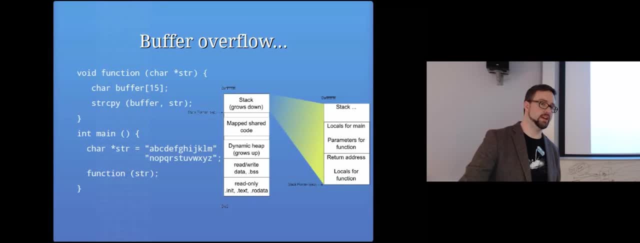 virtual, virtual, virtual virtual addresses for that specific program. so yeah, a buffer flow in your password manager could overwrite the- I'm guessing could overwrite the passwords that are mapped in memory somewhere. but one program can't access another program's address space, so there the kernel restricts access to it. so you, if you've got one program, can't just read all the variables from. 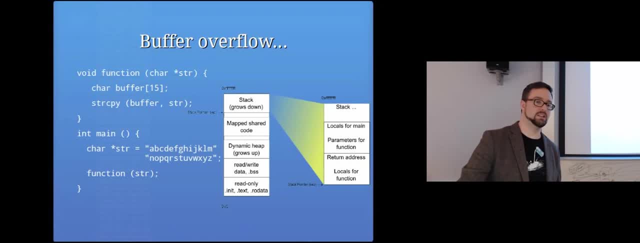 another program, unless you like, dumped the context contents of ram or something. but that's what what you're talking about is supposed to protect against. so if you're using protected memory and stuff, then I'm assuming it. it doesn't just store it in ram, um, but yeah, I don't know specifics. let's. 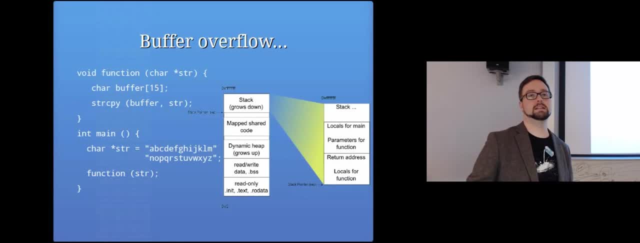 talk in my head: yeah, so well, that's a. with programming languages that are saying they just don't do that level of stuff. I mean the, the C code gets compiled down so assembly code that matches very closely to the code. there's not a lot of extra protections and extra checks that get put into point. that I'm 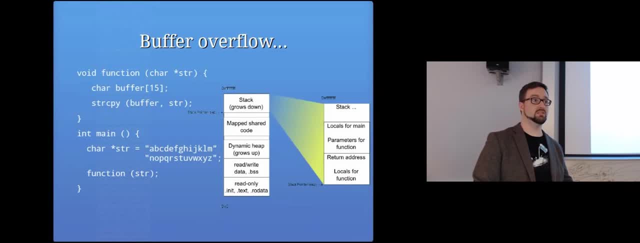 place. basically, you're looking at the c code, which is almost represents the assembly. it's like it's assembly language. uh, is basically the, the exact bare instructions that cpu is processing. uh, so the machine instructions c code was invented in order to create the unix operating system. 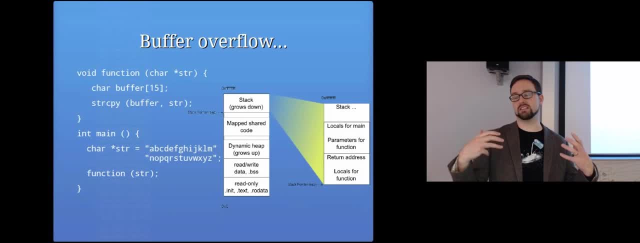 and it was literally. they had something written in assembly. they wanted to create something that's this higher level language, and at the time it seemed like incredibly powerful tool to go from looking at these machine instructions to suddenly talking about these high level things like a for loop or something like that, like it was very um was great at the time. 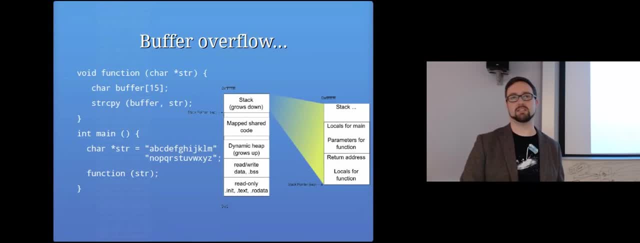 but they it's not at the level where it will check variables, types and things like that and the compiler will do some checks, um, but not the the extent that what you're talking about- newer programming languages- do put those kinds of checks in place, because there's a whole lot of 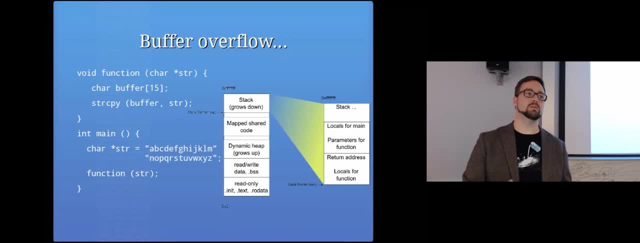 extra code that happens other than the actual code that you write. so when you compile a java program, the the java itself is like a virtual machine that's doing a whole bunch of extra stuff like collecting that memory out, memory management and all that sort of stuff, whereas if you're using c 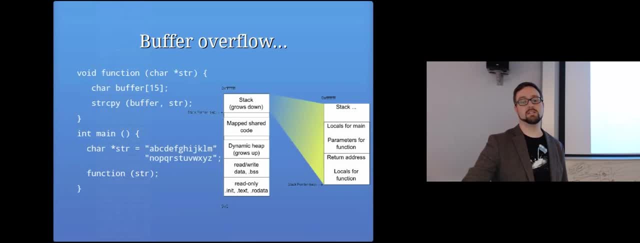 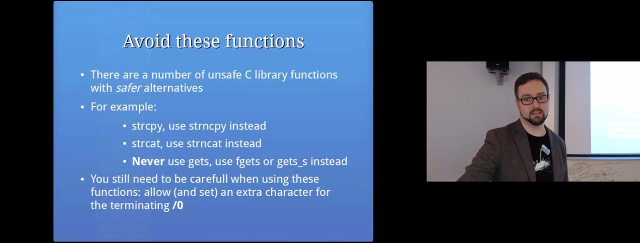 or c++, you actually have to do all that itself within the code um. so, yeah, it's, it doesn't protect against that um. any other questions? yeah, i think. i think that. that. um. it's probably a lot clearer to you now how the buffer overflow works. so if you want to avoid making that program mistake, there are a couple of things you can do. 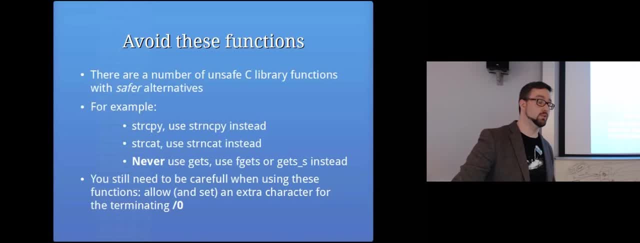 well, you could. basically you could use a different programming language. that just kind of helps you out in that regard. but if you're using c- and in a lot of cases you have to- for example, the entire linux kernel is written in c. a lot of windows stuff is written in, like. quite low level programming languages. if you're doing any systems programming, c is the way to go, basically, or c++, um. it's a very fast because it doesn't do all those extra checks and everything. as a result of that, very, very efficient um code, um plus, if you've got existing legacy code that's written in c, then you know you're stuck, you're. 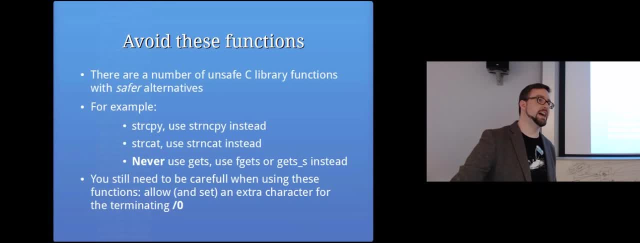 stuck with c, but so if you are writing code you can use functions that provide the checking for you. so instead of using stir copy, so string copy. use string and copy um, which will um as one of the parameters. you say how much to copy from one place to the other, so you say: copy this. 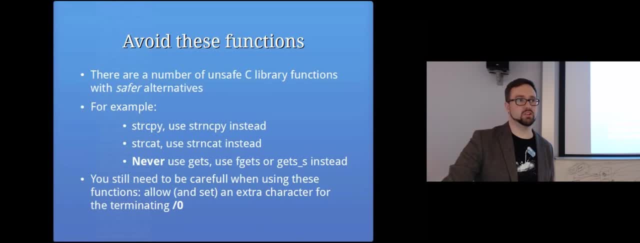 to here and copy up to 10 characters and then, if it hits the limit before it finishes copying the string, it'll stop. um so same with string cat concatenate. so stir cat, use stir n cat instead. never use get s, which is the example from last week. um use f get us or get us underscore s instead. 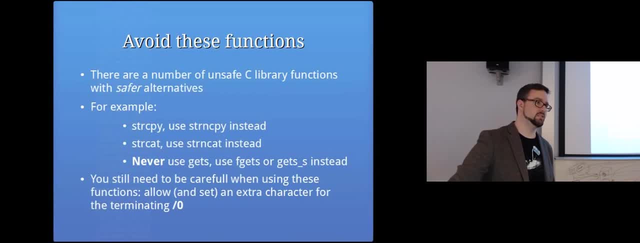 so there's, there are a bunch of newer implementations of these um library calls that will provide the checking for you, so you just have to tell it. okay, this is how, when you call that function, you say: don't copy more than this amount, and it'll make. 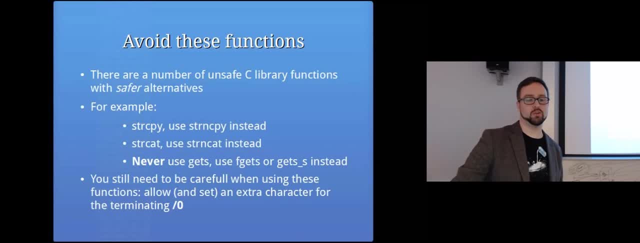 sure that that doesn't happen. uh, you do still need to be careful because there are some weird things where, um, it might say you tell it there's 15 characters, it'll copy 15 characters and then stop without actually writing the null character at the end, which means it's the end of a string. so 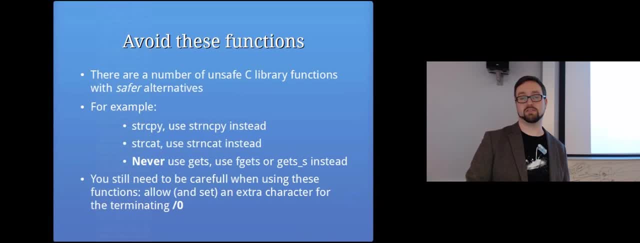 you just need to be careful to read the you know the manual page or whatever for the functions that you're using. so you know, in the man pages that you guys know so familiar, you're so familiar with now in linux, you can also use it to look up pretty much any c function. 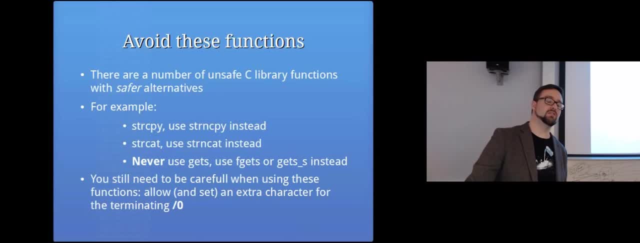 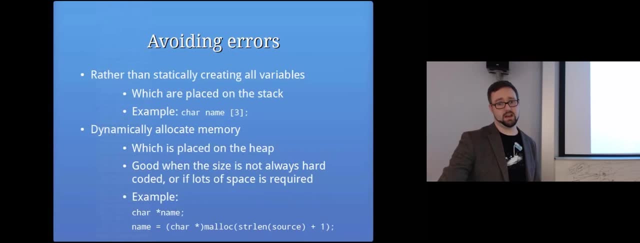 because it's all documented in the man pages. but you do need to check those sorts of things, so like whether it puts the, the um, that null character, at the end of a string for you. um, so if you declare all of your variables statically, so as in, you've got your function and then you 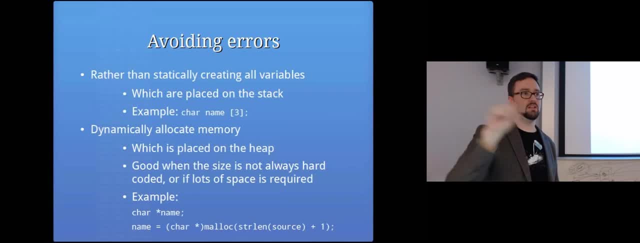 just declare all your you know into this. you know all that sort of stuff, and then it gets put on the stack um instead. you can dynamically allocate memory instead, so that ends up in the heap instead of on the stack um. it's good if this, if the size isn't hard-coded, so, for example, 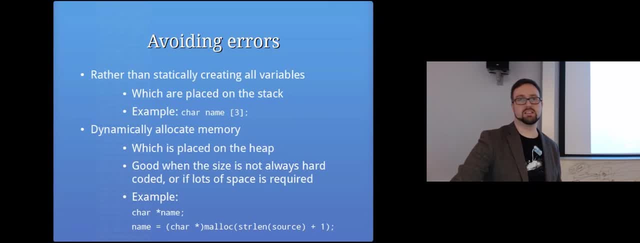 you want to read in something from the user, but you don't know how long it is, then the heap's the place to go, really, because you can just allocate more and more memory, whereas the stack is has a limited size, um, and you can, you know, only allocate a certain amount, so sorry. so how could it, uh, keep allocating them? 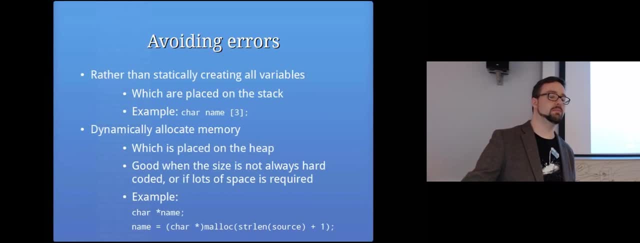 yeah, but the the space is quite large between them, but there is, there is a limit, but probably not as much as your ram is a limit. so there, there, there, there are limits, um, but you know, as long as you've got enough ram, you should be fine. so here's an. 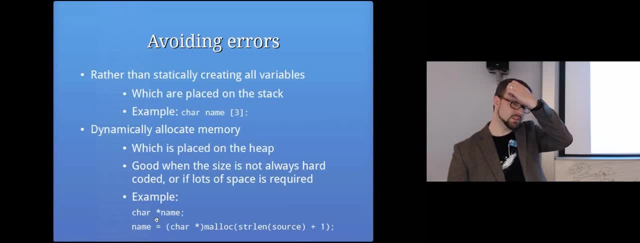 example of some code where you're dynamic, dynamically allocating. so here we've got a char, star, asterisk name, and the asterisk is a pointer. so a pointer is just a. rather than storing the thing itself, it stores the memory address of the variable, so where it is in memory. 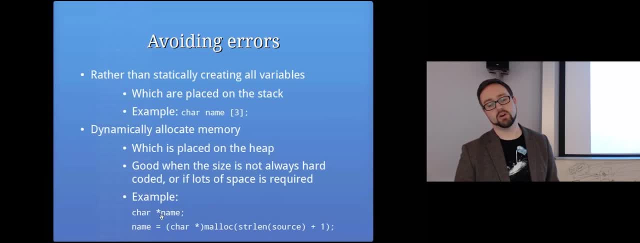 so so we've got a um, a pointer for characters called name, and then here you can just say: name equals, and then that's just saying, store it as a character pointer and malloc, so allocate memory, uh, and then you tell it how much memory you want. so in this case it's this the length of the string. 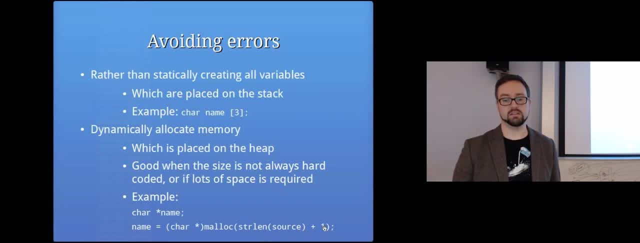 plus one for the um, the null pointer at the end. so, and then that will basically allocate you some space on the heap, and then this name will then be pointing at that space in the heap rather than just saying um. you know, in my last example chart, um name equals and then just declaring it up in this on the spot, which would end up on the stack. 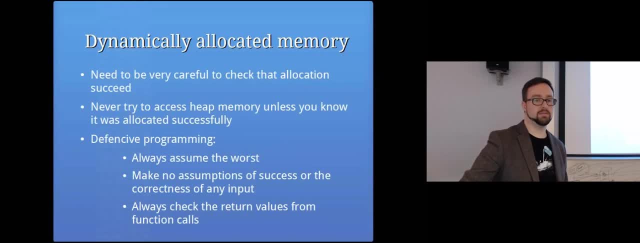 um. so you need to be careful, like all these things in to do with security, that you check the return values of everything. so when you say give me some space from the heap, um, you actually need to check that the re it succeeded and did give you some space on. 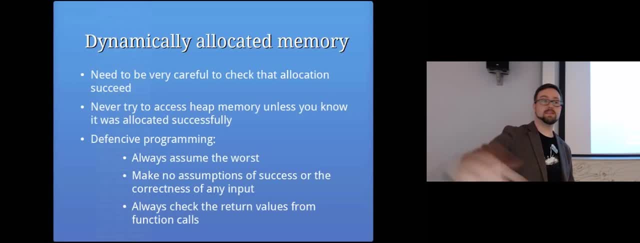 heaps. so say, for example, you did run out of ram or something and you said, give me more space, it might give you more space. and then you say no, it failed. and if you don't check that in your code, did it succeed there and you just start accessing it. that can cause security problems, because now 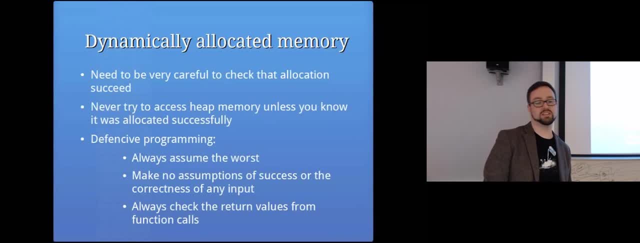 you're reading and writing out of somewhere that hasn't actually been allocated, memory that's not allocated, and usually you know the good case scenario is that it just crashes. worst case scenario is something worse happens, um. so yeah, basically everything. when you're programming, if you care about security, just be really careful. check the return values of all the. 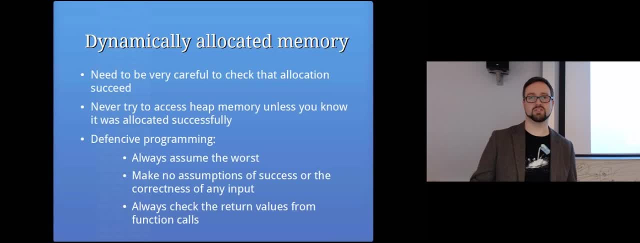 functions. so if you call a function that says it can do something and it has a return value that says whether it succeeded, just do. if you know it succeeded, then do this. otherwise you know an error message or something. it's important to actually check those values. so here's an example. so the 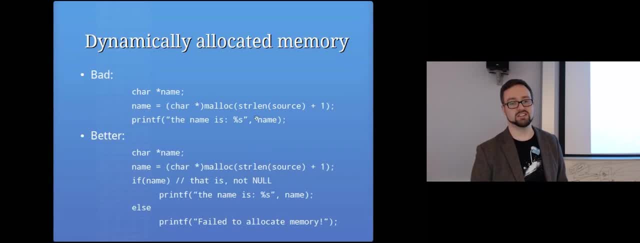 bad example, like on the last slide, where i basically just did that. if you then just started using it, yeah, that could go wrong, because actually we don't know whether that succeeded. so the better solution is to say if name. so in other words, if that variable isn't null, if it. 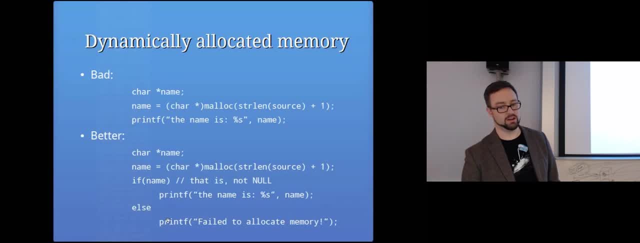 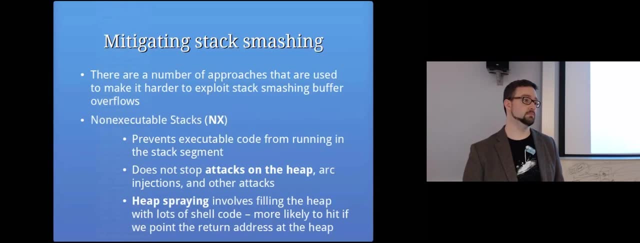 doesn't equal zero, then you know, do whatever. otherwise you can just like give an error message saying failed. you're actually displaying here why it's actually failed. um like in this case, it's probably probably not much of a threat to know that you've run out of ram in some. 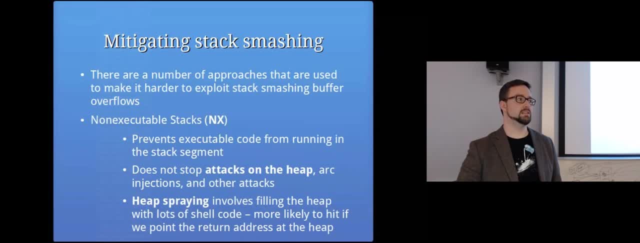 cases you're right. if you are talking about developing a website, for example, and you tell the user lots of details when something fails, that might give them insight into your website that you don't want them to have, but in this case i don't think it's a threat. so, for example, say something. 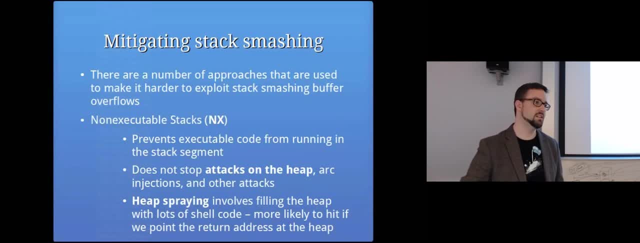 failed and you told them the names of all your tables in your database, then that wouldn't be good. but if it in, if it's just run out of ram, like memory there's not really. i suppose worst case would be they looking at if they've got access to your code and they might analyze that. what can they do if there's low memory use? 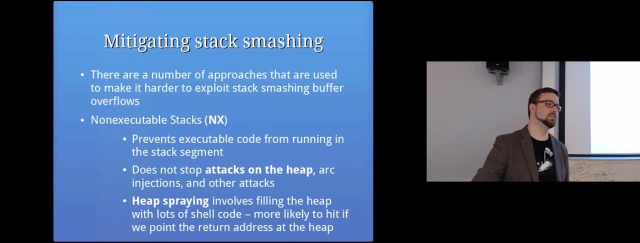 and maybe there are those sorts of mistakes that we just talked about that they could take advantage of, but very unlikely. you know, like blue post effects happen when people know where, where you're running out or where you're, you know, uh, you know dead ends, and then they try to just 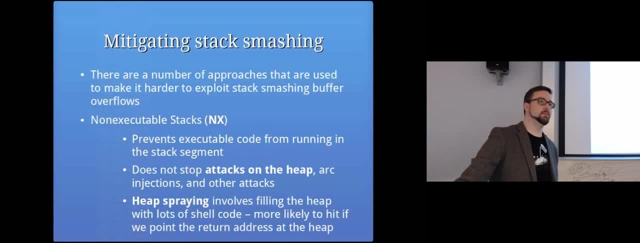 yeah, like there, there are some cases where you want to limit the amount of information that you provide to an attacker. um, yeah, okay, so there are some things that that researchers have done and are available in various operating systems that can try and limit this damage that happens with. 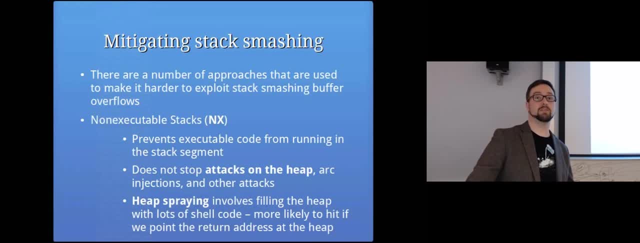 buffer overflows because it's so common, like buffer workflows, are just ridiculously common. people like to think that these things will actually help them. they don't need to be able to make these kind of mistakes so easily. like you know, it's really easy to just, you know, get the. 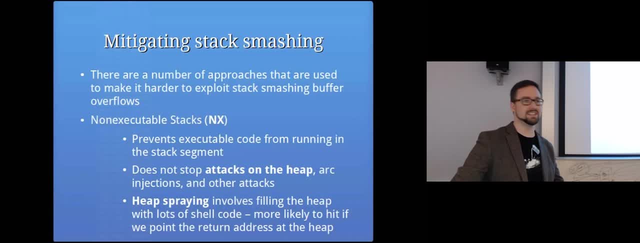 number wrong or you just you don't think about the fact that you're writing into somewhere, and how much should it be checking? and a lot of programmers don't have much knowledge of security. basically, they just they write code and does it work. oh yeah, cool, i finished um, where you know. 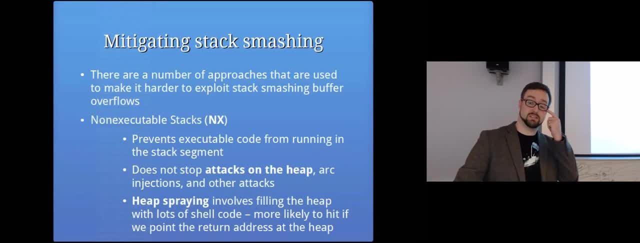 whereas we know that actually it's very easy to make a mistake. that causes big security problems. so in order to combat that, there is a number of things you can do. so one of them is to use non-executable stacks, so you basically say: any code that's in the stack, you can't run that code. 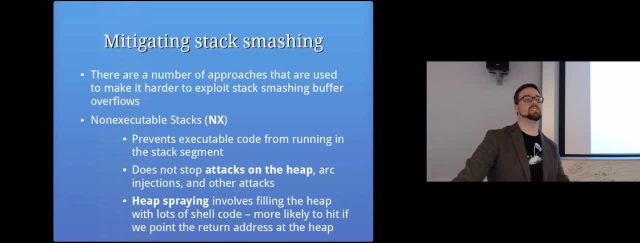 you can have variables and you can have data stored on the stack and the program can access and write to that memory. but you can't just have machine instructions sitting on the stack. um, again, this doesn't actually stop attacks on the heap, which also happens. um, sorry, did you have your? uh, no, um, it doesn't stop arc injections, where you basically just 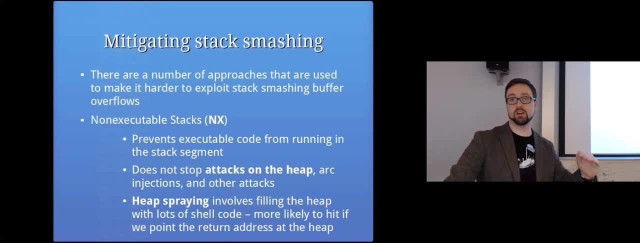 jump to somewhere within the program, somewhere else within the same program in the code um, and so there's a whole bunch of stuff that doesn't stop um, but it does stop. it does make buffer overflows a lot harder, um, and in a lot of cases, on a lot of offering systems. that is now the case. 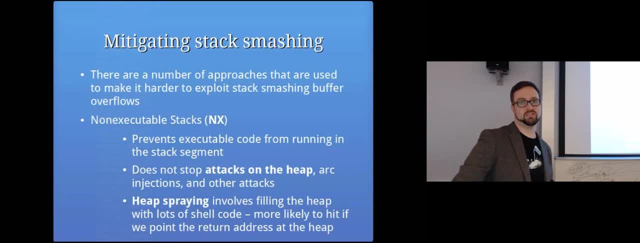 where we've got non-executable stacks. if you use older versions of any of the operating systems that you know of, they probably didn't have non-executable stacks, and then it's a lot easier. yeah, um, um. so you think that if we say that you're going to the security? 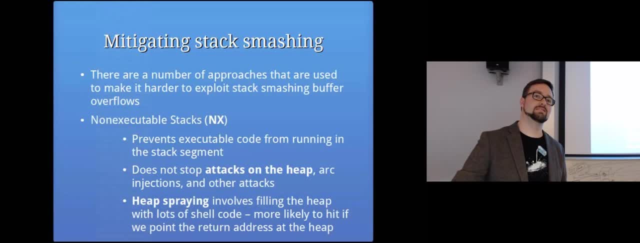 i already think it would vary in money from the fact that you have a security mindset. that's going to take you a long time to be able to develop security at the end of the day. um, it does take longer when you're doing things properly. um, it's true. so so the question. so the question was like: if you 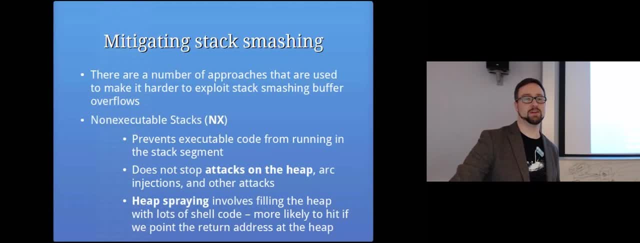 have all this knowledge and you've. you know you're working as a software developer. aren't you going to annoy everyone by being really slow at everything that you're doing, because you actually care, uh, and writing good quality code, and that's true, um, that if you are working in a big enough company. 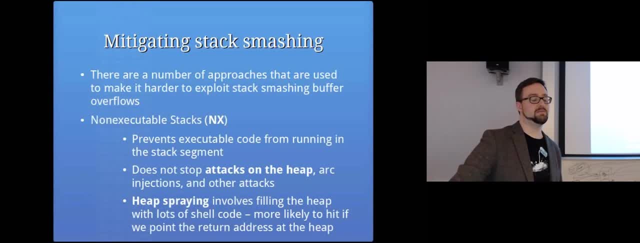 they should value and respect that and in fact, most companies that are large software developer companies will have people who specialize in the security side of things to try and train other people in their organization to look for the you know the problems in their own code. um, it's like these software. 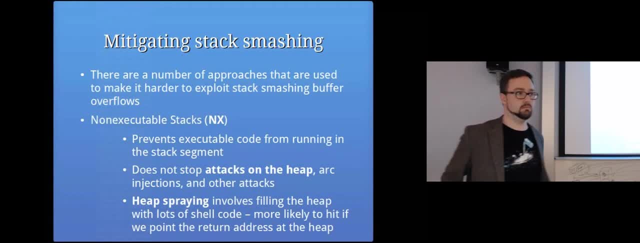 customers in manchester. you know all these shows. basically look at all the softwares that they program there for the test on them, checking if there's any leakages on them or doing feasibility checks, and apparently it doesn't. you know what you're supposed to do, or not. 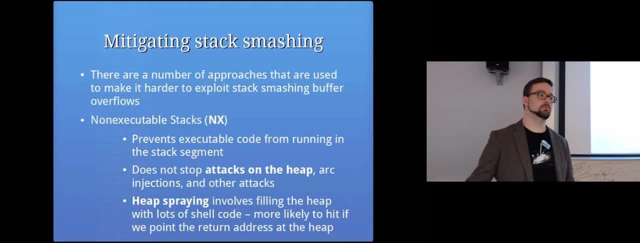 I guess you know that's what they do with people. even if you know you're the best programmer and you know the security, still they should be over here first. you should always test your code and I'll talk about that next week, but um, yeah, it is important. 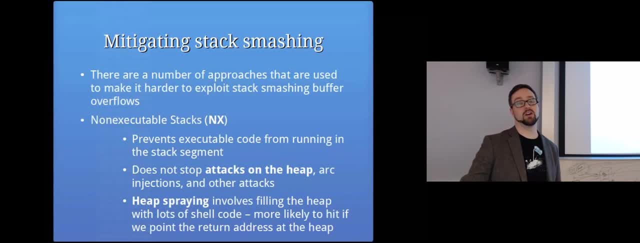 and it takes a bit longer. but I guess the more that you do programming, the quicker it gets. it's just a matter of checking, you know. usually it's basic stuff like checking return values. it's not hard. it's not a hard concept, it's just that. 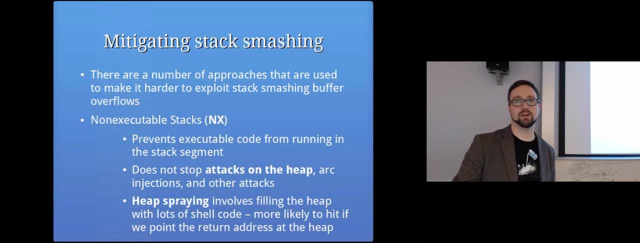 when you're lazy or even something. if you're looking at stack overflow example code and stuff like that, they often don't. if you're just copying, like you know, a lot of examples on the internet are bad and they're not good examples, um, but if you just look at the documentation, 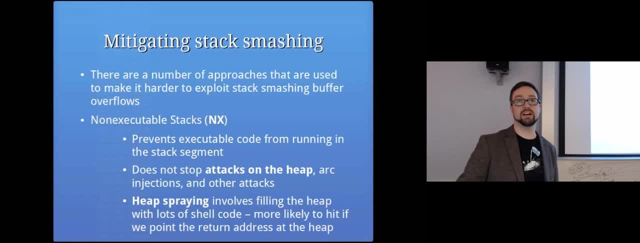 for the function you're calling. what does it return? does it return a status value? check it. there you go. it's one extra line of code, um, but it's gonna potentially save a lot of heartache in the long term, um. so another type of attack is heap spraying. 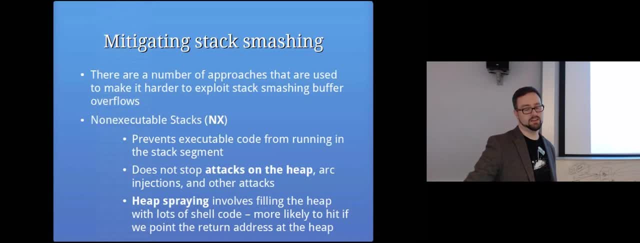 so basically you fill the heap with lots of shellcode and then jump somewhere into the heap and hope that you hit it. so it's a little bit more finesse than that, but basically, if you um, because the heap is dynamic, you can just keep asking for more and more space on the heap. 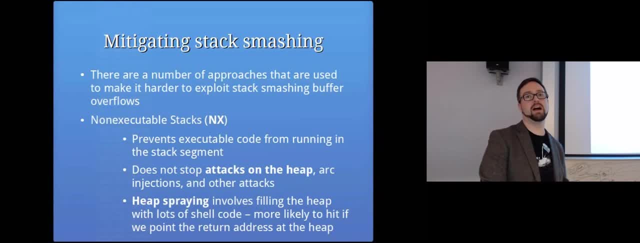 keep putting shellcode. you know if you might have, um, for example, javascript code or something you know like in a website and you might be able to just keep calling that function that loads a variable with some shellcode, and then, if there's some way of pointing, 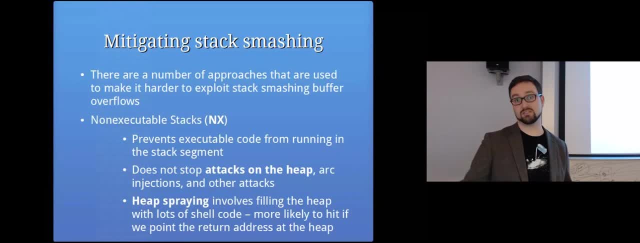 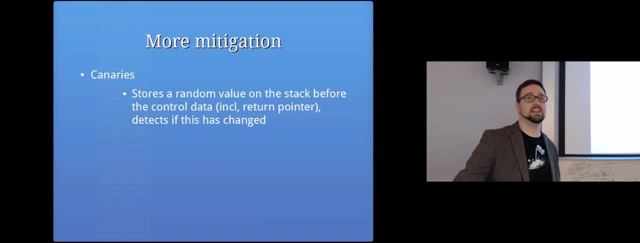 the um, you know the instructions straight into that heap. then that you know that might work and you hit one of your shellcodes and then you've got um, you've got yourself um shell on that, on that machine. something else you can do is what's known as a canary. 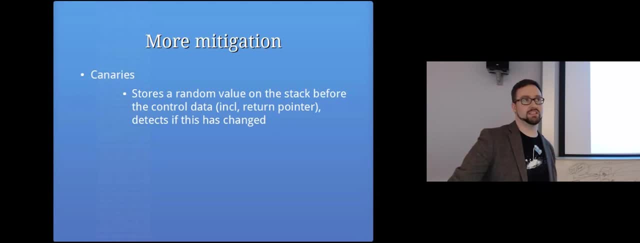 and um, it's kind of what it sounds like. i guess like it's a way of checking whether well, i guess, if the canary dies, then you know it's not safe. so basically you store some random value on the stack before the control data, so before the return point, you. 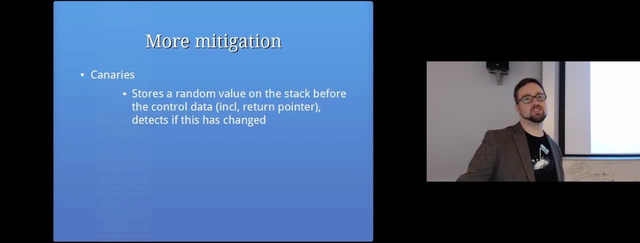 put something on there and then, before when you're changing back- you know, moving to back into the previous function- check that the canary is still there and as it was, and if that's true, then you know that the buffer overflow probably hasn't happened, unless they're clever enough to. 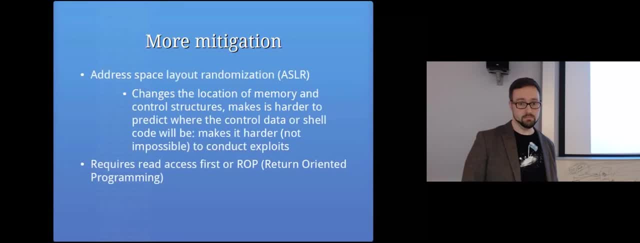 know what the canary is and put it back um. so that's another technique, um. the most common defense that is now in place on most operating systems, including linux and windows, is um address space layout randomization. so a s l? r. and what that does, is it? basically it. 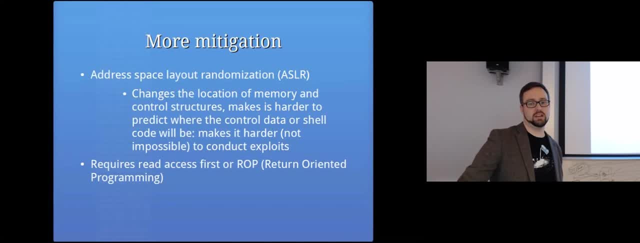 randomizes where things are in memory, so it'll move around things like where the stack is and where the shared code is and things like that. um, which means that if you're setting the pointer somewhere else, if things keep moving around every time you run the program, it's harder. 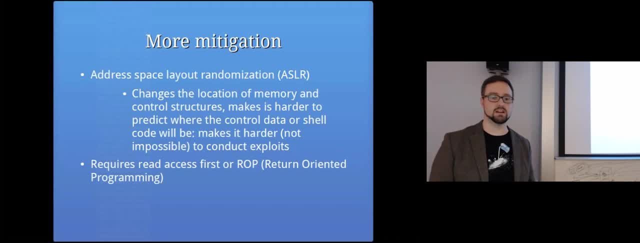 to point, to point it at the right spot. right, because it's like a moving target and then you need to use, like either look at things first if you've got some kind of read access, or use something known as return oriented programming, um, but basically it does this. 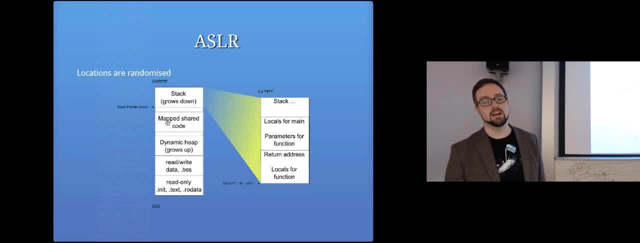 so this. so this is our picture again of the stack and all the memory, and so this mapped shared code might move around slightly. each time you're on the program the stack might move slightly, you might have the heap just like somewhere else in memory. so just like kind of moves. 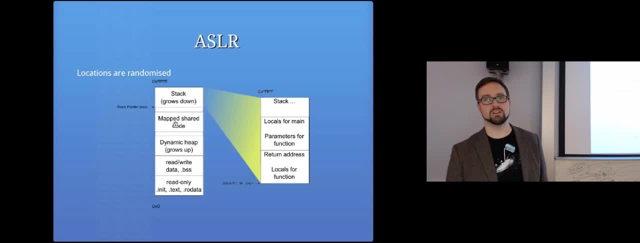 things around a bit, which means if you're jumping the pointer somewhere else, it's harder to hit the right spot, and those are things that we'll look at how to get around, uh, in a little. in a little bit, um, in a couple of weeks, yeah, you know. 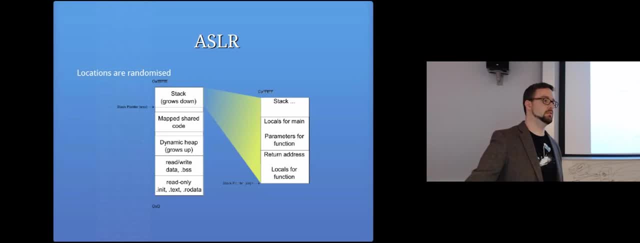 in linux you've got built-in thing that if your ram reaches maximum, you know it just crack kills all the programs, the ones which i think overload or something. okay, yeah, just wondering, you know, if you're using something like this on that, what? how would it go around? because 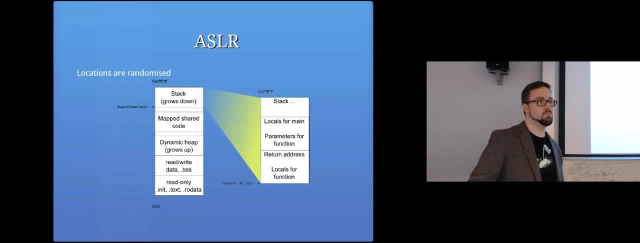 um, i'd be surprised if that's true, saying if, if a program manages to use up enough memory, the whole computer will crash. no, no, no, not a program, but if, uh, you know all you know programs that use the whole of the linux memory. yeah, one of. 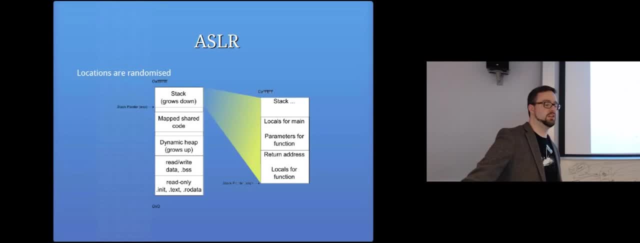 having done some kernel programming. one of the challenges of writing code for the kernel is the limited stack space. so, um, you've only got a certain amount of this. the stack can only grow a certain size before you know for the whole kernel. basically, you know if you've got. 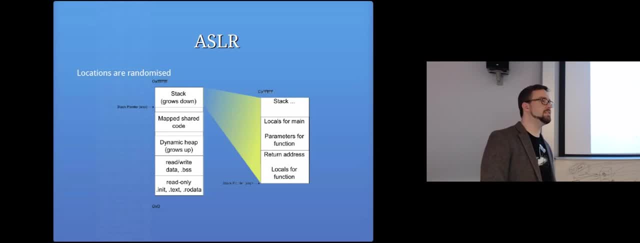 code running in the kernel. you can't use too much stack space. but other than that, i wouldn't uh. yeah, i don't know, maybe because, um, i was only asking because when i used to uh, i used to manage hosting services and on the linux servers, yeah, the 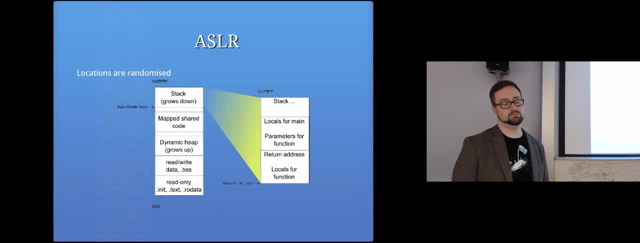 servers will also excel just for all the flows of when, when the amount of time is actually used. well, you know well that is. are you sure you're not thinking of php feature? because php is very um, very strict about memory usage and it won't allow any script to use over like. 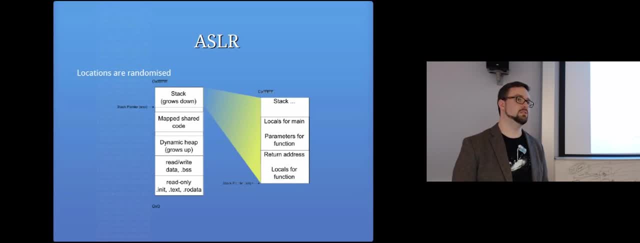 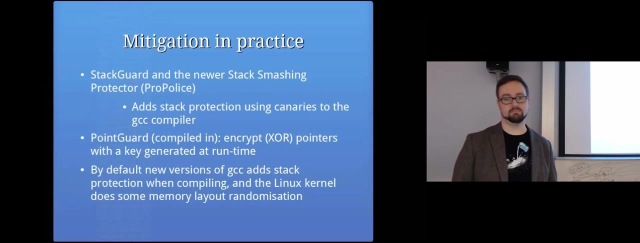 128 megabytes or something by default. yeah, i, just i that might be what you came across. it's got nothing to do with the actual programs, it's just: yeah, all right, um so another. so, speaking of those things, in practice, what actually happens? so stack stat guard and um pro police. 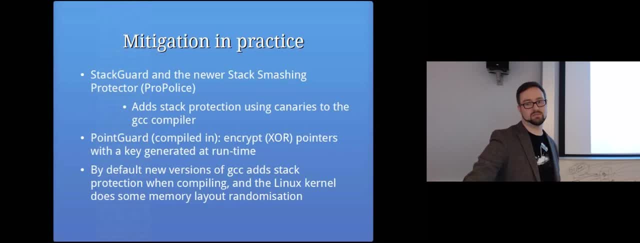 will basically add those features to a program. if you're compiling with gcc, you can ask it to do that. point guard um will encrypt pointers um with a key generated at runtime and by default, new versions of gcc at add some level of um. so that's a little bit of a. 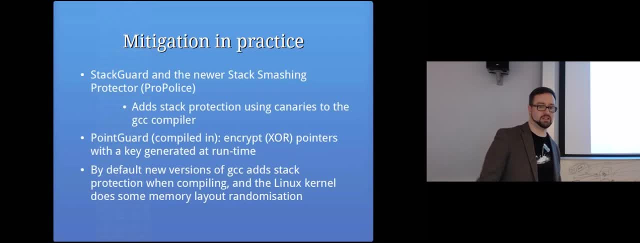 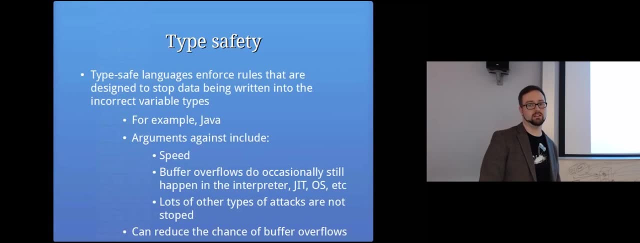 stack protection when you compile and the kernel does memory layout randomization. um. so you know we've talked about type safety now quite a lot. so, um, it is still possible to get buffer overflow on something like java if it happens in interpreter or on the operating system, but it's. 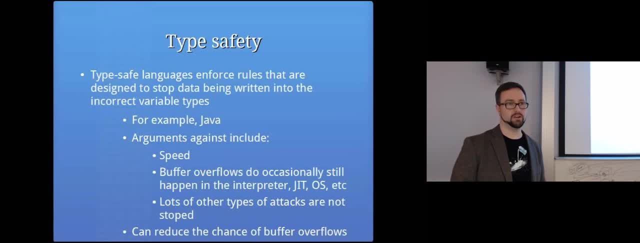 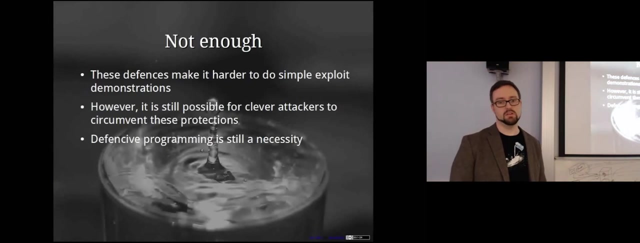 much, much harder to do, much rarer, although a few years ago there were a number of buffer overflows in in java itself. but you know, but they're going to it's. it doesn't happen that often, um. so yeah, as i said, it can help. so all these things make it a bit harder. 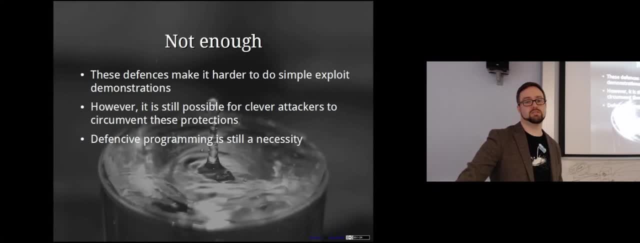 to do like really simple demonstrations of buffer overflows, but they don't stop buffer overflows. there's still. it's still possible to get around these things. um, and you know as you can, the actual, if you look on exploit db, it's just the number of. 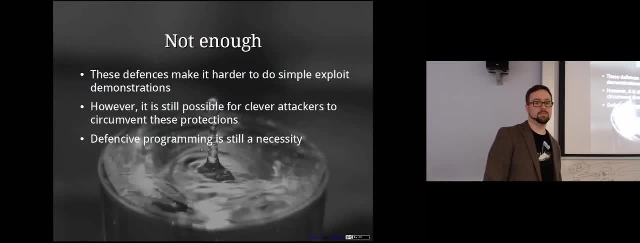 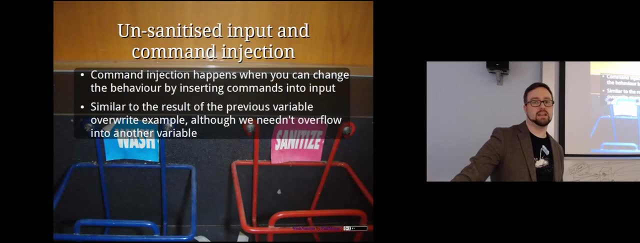 buffer overflows. obviously it hasn't hasn't fixed the problem, so defensive programming is still really important. okay, so unsanitized input and command injection. so command injection is a type of vulnerability that happens when you can change the behavior of a program by inserting commands into the input. 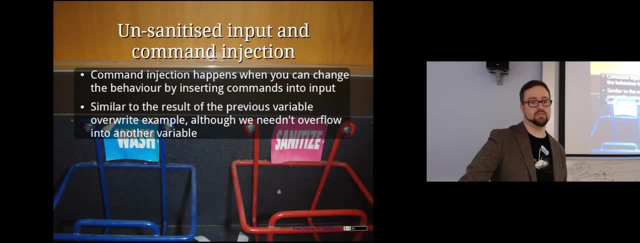 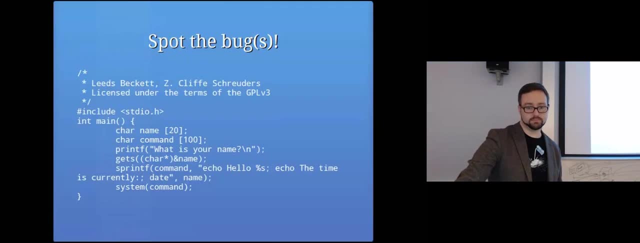 so similar to last week when we over wrote a variable, except that we don't need to actually overflow into another variable. so if you look at this example code here, we have a bug um 10 seconds. if you want to try and spot the bug, uh, yeah, ignore that particular bug. 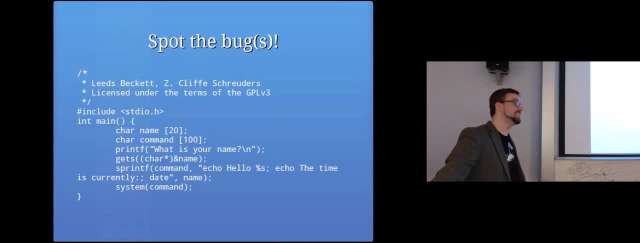 there's another bug in there. you're right. you are 100 right, though get s you should never use. so there is uh, not only is there a buff, potentially buffer overflow, there is another bug. so we're going to do a little bit of testing to see if we can get a better. 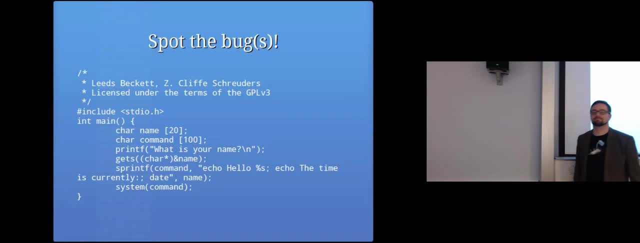 result. so if we can get a better result, we're going to use a, this semicolon here, not far off, no, okay, so, um, so, yes, so what this is doing is it asks for a name. it stores that using get s, which you should never use in the variable name. 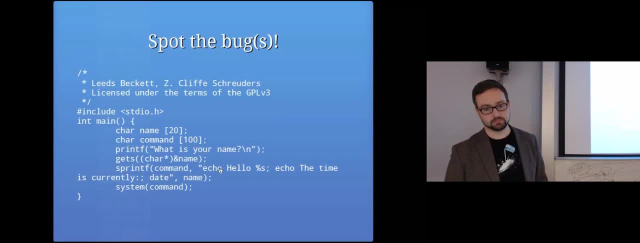 and then it uses printf to um, basically sorry s- printf which writes to this string. so it's putting together this string into this variable, so saying: and you're going to end up with a string that says: echo: hello salmon um semicolon echo. the time is currently. 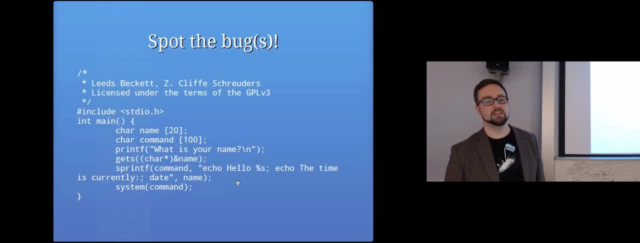 colon semicolon. date end quote: um, any can does that help anyone pick up what their problem might be? and then we take this, this string that we've just put together, and we run it through bash, and then is it: undetectors in there. it's supposed to be in the. 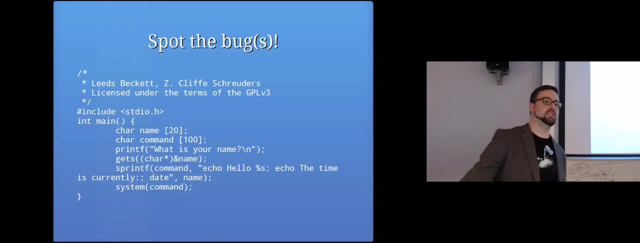 command in the command side of it. no, it's not related. no, it's not. it's not a programming mistake, it's not a. this code runs. it just doesn't do what you want it to do. okay, so the problem is that we are just putting this. 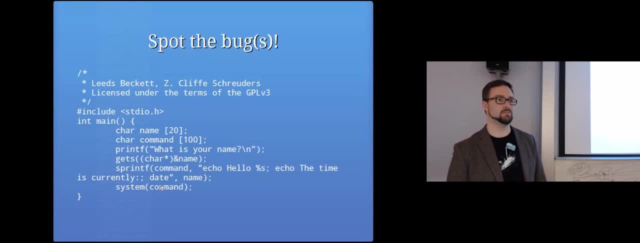 the input from the user into this string and then passing it straight to bash. so the user gets to control what. that is right and you know it says echo. so this is just getting printed to the screen, um, but there's nothing to stop them from typing in. 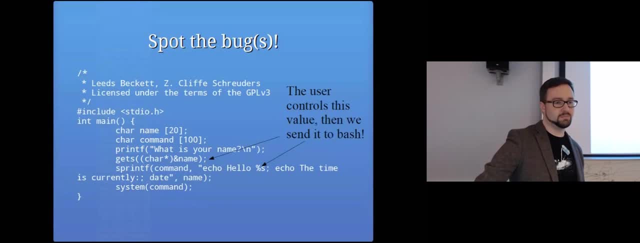 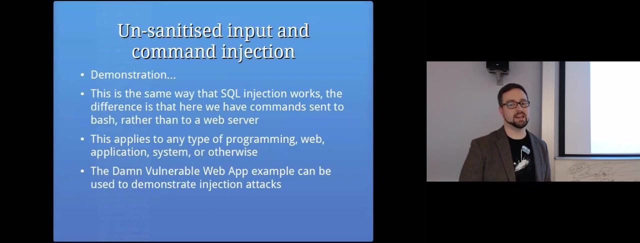 semicolon rm minus rf space slash. just delete everything on the computer and then that will run through this command and, depending on who this you, which user is running this program, bad things will happen. so, um, so, you're going to be able to do a lot of things, um, so, yeah, it's the same. 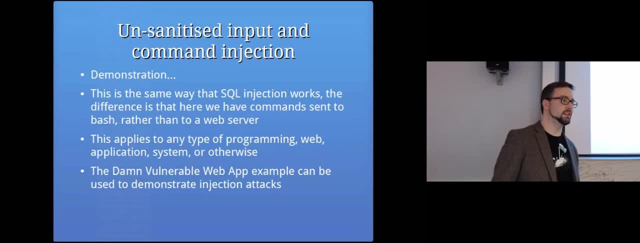 as how sql injection works. basically, the difference is that we're sending commands to bash rather than through to, you know, the database on a web server. so, um, basically any type of programming language could this could happen. so java, c, sharp, um, whatever you, whatever you want to use. 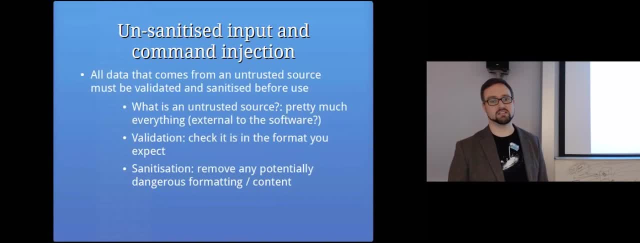 if you use the damn vulnerable web app, you can get some, some nice examples of injection attacks and so basically, any data that comes from an untrusted source. you will get a lot of data. you really have to validate and sanitize it before you use it. so what's an untrusted source? basically? 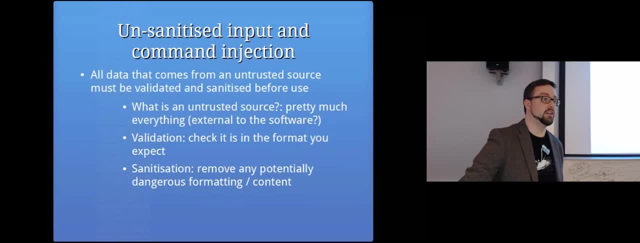 everything. um, if it's coming from outside- the software, a file of a computer, a network connection over the internet- then you need to to check. so you do check validity, so actually check it's in the form you expect and and or sanitization, where you actually get rid of anything that you don't. 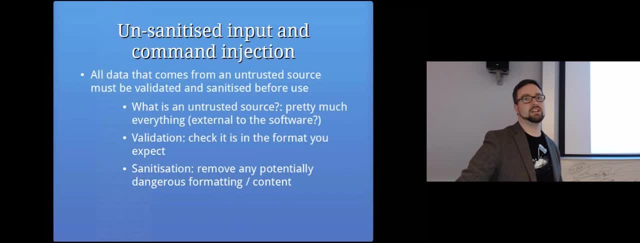 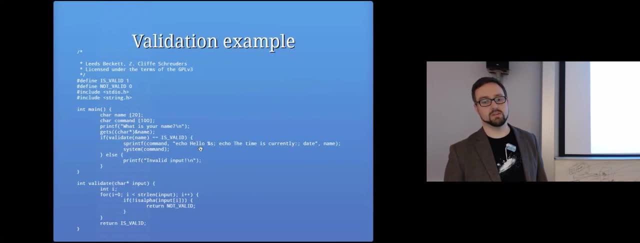 expect. so if they enter something and it includes a semicolon, get rid of that semicolon. and get rid of that semicolon, then you can get rid of it. so, for example, so here's an example of some validation, we've got some code and, um, basically, we check if the name's valid. 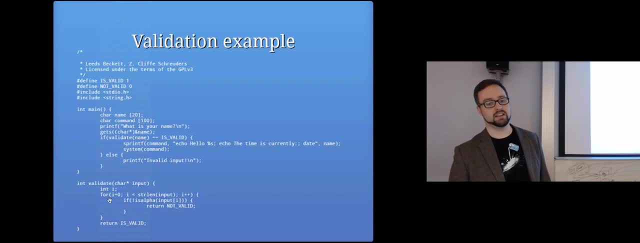 before we then print, do that command and we do we, and otherwise we'll just say it's invalid. and this validation basically just hit a for loop and just checks every character to find out whether it's um is alpha. so is it? is it basically output um a letter? if it is, 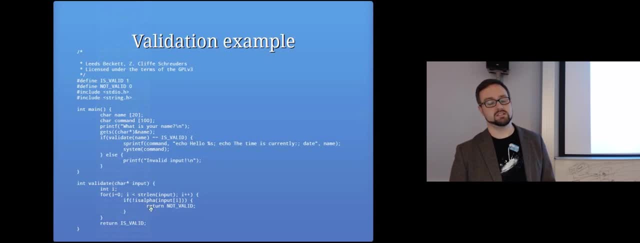 it's fine, i'll get to the end and it won't be a problem if it hits something. so it's not a letter. it'll basically return an error and then it'll will refuse to type out. you know, run that command, so that's, that's validation. so 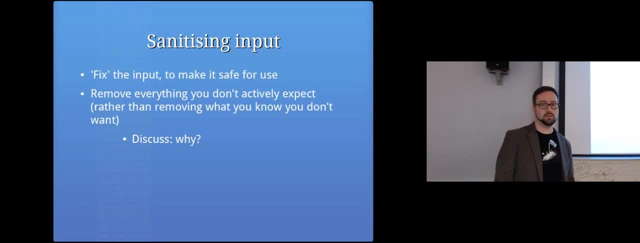 sanitization will fix it um, and basically get rid of what we're not expecting um. so what do you think the better approach is? do we get rid of everything that we can't think of could be a problem, or do we just? or do we get rid of everything that we um? 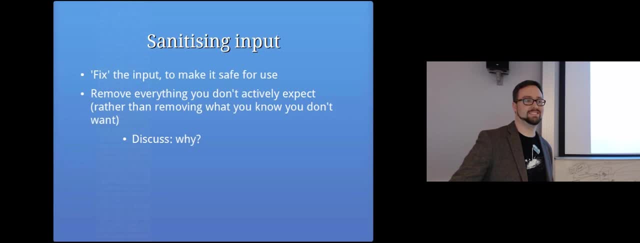 you know that isn't what we're expecting. okay, one, how important security is in that application doing what you're wearing? if you know you're just expecting the name, yeah, then you can say that if it's a an application where they could actually be potentially writing an example of 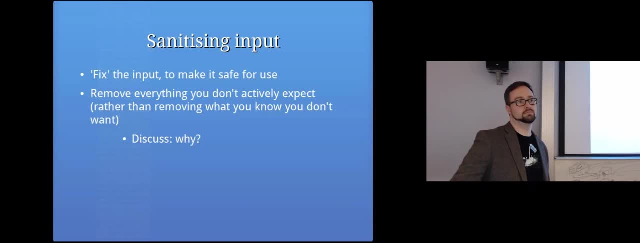 code is there, then your application would work. yeah, well, yeah, okay, that's true, but you, you just need to think carefully about the things that you want to allow. so if you want to allow code, then you need to allow it, basically. um, yeah, chris, would it depend on? 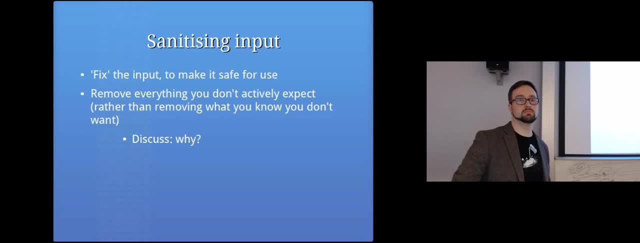 your knowledge, you know situation that says yeah, yeah, yeah, yeah, yeah, yeah, it's yeah and you're right. it is context of the application and what the security problems are that it faces and all that sort of stuff. but in general, if you have to choose between having a list of 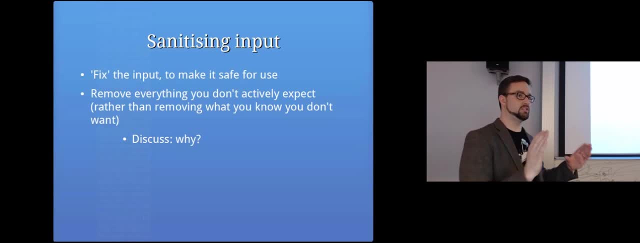 characters you'll allow or a list of characters you'll deny. it's better to choose the have a list of characters you'll allow because there's a way to do that, because if you say okay, i'm going to allow all you know, if it's a name, i'm going to. 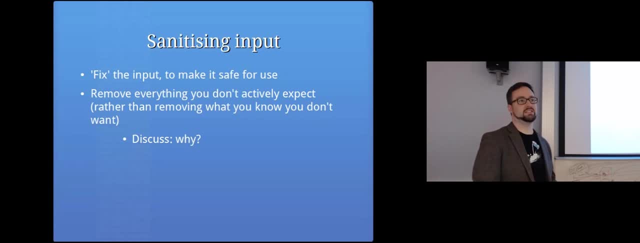 allow all the letters in the alphabet. you know, worst case scenario: someone has an equal sign in their name or something which you may have had on your student records for some weird reason, um, but i believe your name doesn't actually include an equal sign. um, but it will prevent. 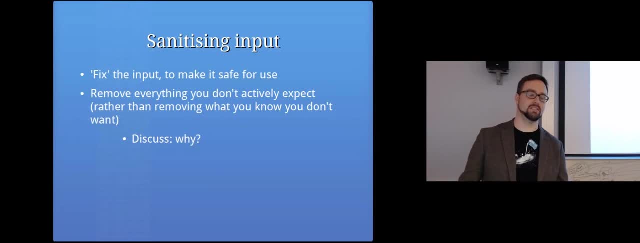 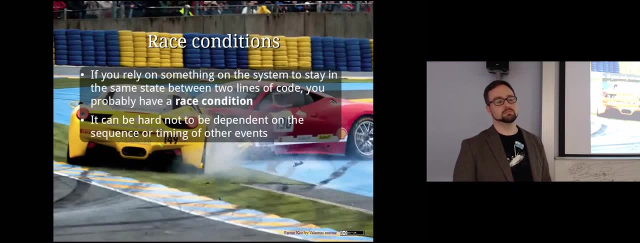 all sorts of problems from happening in the future if some people are processing that information. but yeah, just like i think passwords, isn't it some some place? if you go for a password, they just ask you just a lower and a small character, and then sometimes you ask me for a digit. 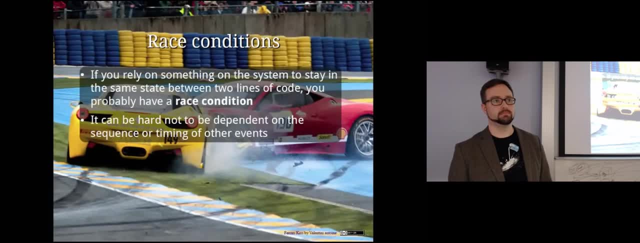 with it. but at some place i would say you have to put a character and part you can only put. you know these characters you know, otherwise you know the password doesn't work. so you have to put like a dot or something like that. yeah, okay, so we're running out of time, but um, 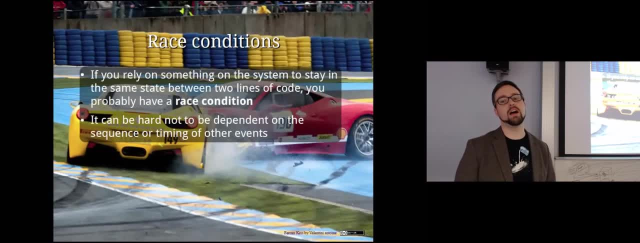 so race conditions is where you, if you rely on something to happen in a certain order, or if you rely on states staying the same on the computer between multiple lines of code, then the chances are you've got a security problem known as a race condition. it can be quite hard to write code that. 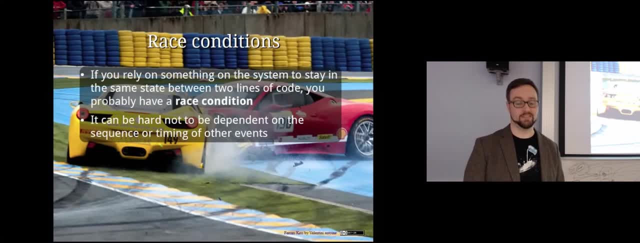 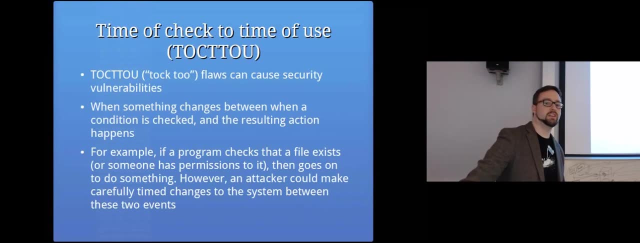 doesn't depend on the order that things happen, right, but it's something that can happen. so at time to check, to time of use or talk to flaws cause security problems and basically when you check if something's true and then you do something, you know your computer can do a lot in a 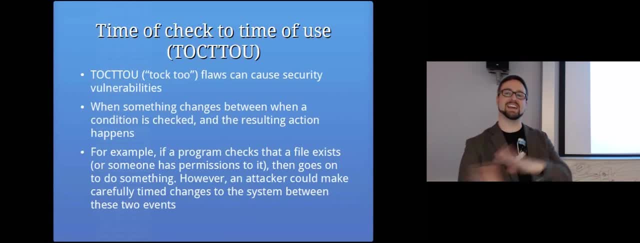 very short amount of time. but if you're doing a lot of time and if it happens to do a whole bunch of stuff, it might actually get in there and do something you didn't expect to happen in between. so you might check a file exists before you delete it, or you might check. 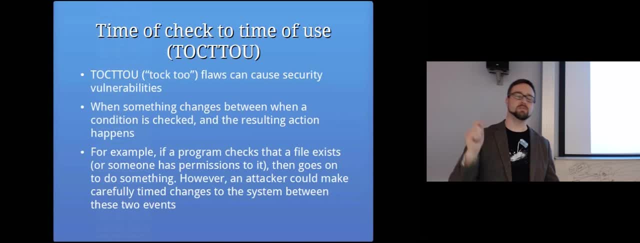 that a file exists before you start writing into it or appending to it or something. but if in between those things happening, someone like deletes the file, puts their own file there, changes the permissions on a file, or something like that, you can end up having serious consequences. so 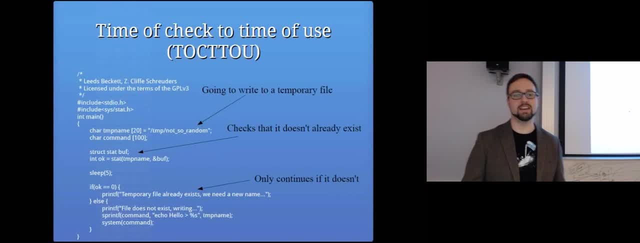 here's some arrows on the slide for you, since you love it so much. so we've got here. we've got some code that's got a name of a file it's about to access, checks that it doesn't already exist, and that's what this part does. 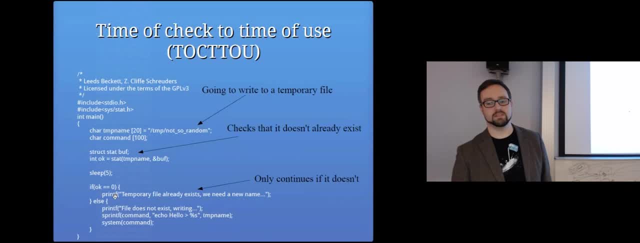 uh, then it. if it um doesn't exist, um then uh, then it will write to a file. so it's checking. okay, the file isn't there, okay, put something there. that's a security problem, because if, in this case, we've got a five second wait, but just imagine you've got something. 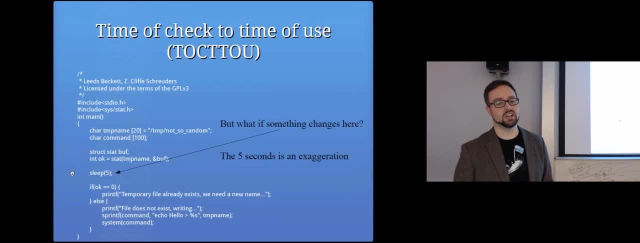 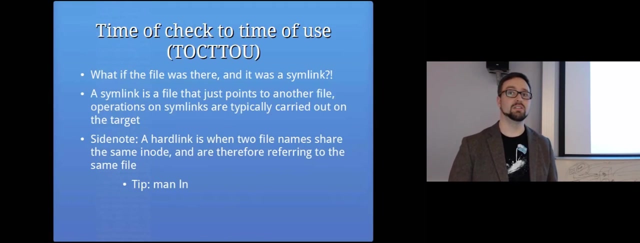 happening in your code here? um, if something changes here, it's going to write into, possibly, a file that exists and cover it, or basically delete a file. that's that's there. um, so what if the file that was there was a sim link to another file, for example, so you might create a sim? 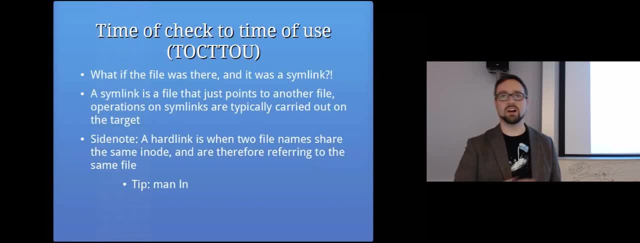 link to the shadow file and then the program writes into it, manages to delete everything from the shadow file and basically, um you know, stops the computer from working. or, in a worst case scenario, you can control what's writing into that file and you end up overriding. you know, the user. 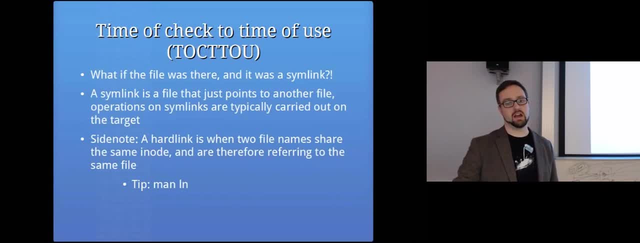 account passwords or something like that. so, um, when obviously a sim link is a file that just points to another file, so any operations on a sim link will actually get carried out on the target. um, and this hard link is when two file names have the same. i node, and so it's. 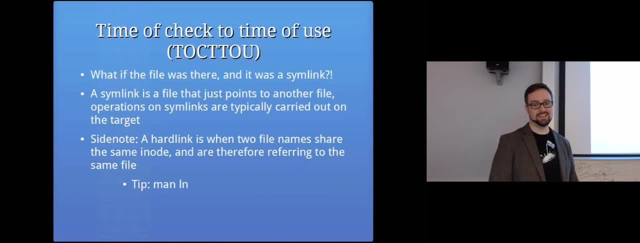 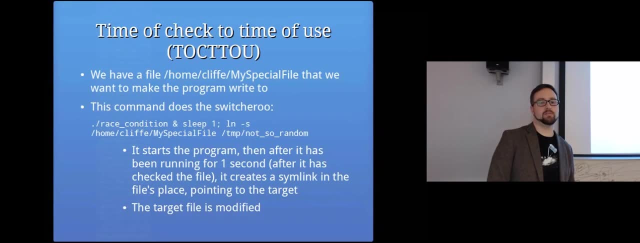 like two file names pointing at the same file. so, man ln, if you're not sure what i'm talking about. so, um, um, if we were going to run this, this program, we have a file named um- you know my special file- that we want it to write. 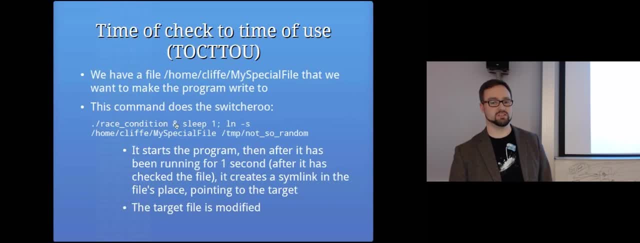 to. we could run this which does the switcheroo: so we run the race condition program, we sleep for one second and then create a link from my special file into some temporary file, um, and then when the program starts, after it's been running for one second, 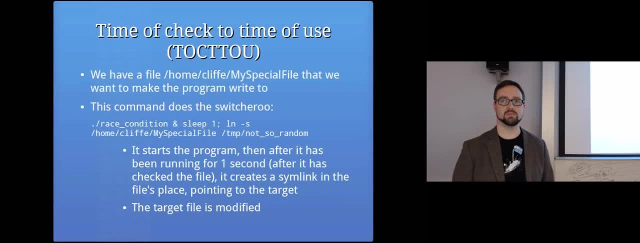 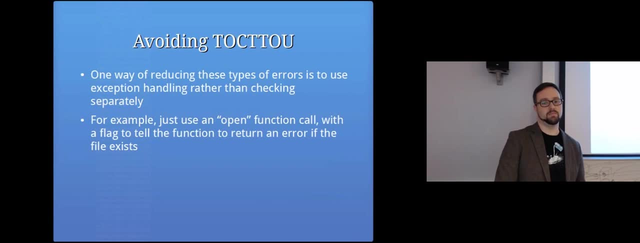 it creates a sim link in the files place pointing into the target, and the target file gets modified. so it's really easy to do. so all sorts of things can happen. so how do we avoid this problem? um sorry, i will not let you stop me because we are running in time. 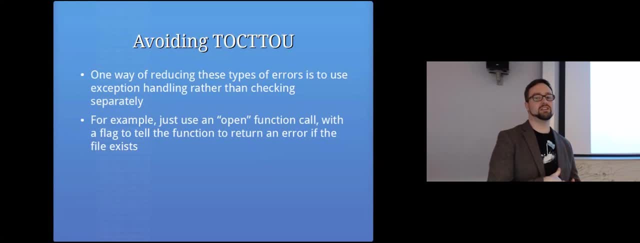 so one way is to actually just make sure we use exception handling instead of checking status and then going on to do something. so, for example, um, you can use an open function call that says open this for writing into a new file, and if you tell it that information and 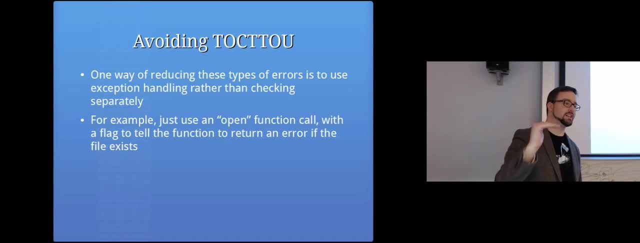 it fails because the file exists, that's. that's something that happens in one step, so it can avoid those kinds of problems rather than checking if it's there and then going on to do something. Instead, you just tell it when you're opening the file what you expect the condition to be, and it will basically tell you if it's not. 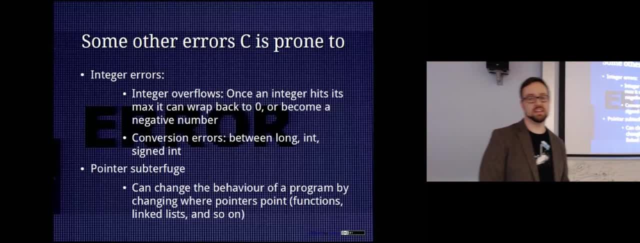 going to happen. So some other types of errors in C. that it's quite easy, is an integer overflow. So an integer is a whole number. Integer has a certain amount of space that it holds a number in. If you hit a number of a certain height, certain maximum number or minimum, if you're going in the 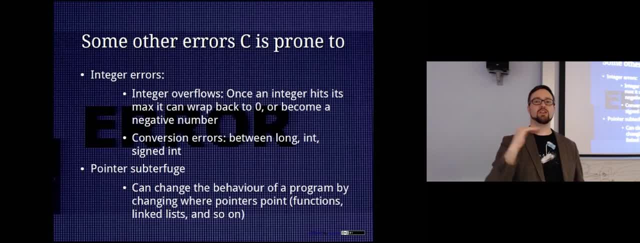 opposite direction. it can actually overflow, so you can go from a really big number to actually a really negative number or, you know, back to zero, depending on if you're using a signed integer or unsigned. so whether you include negative and positive, So you can get conversion. 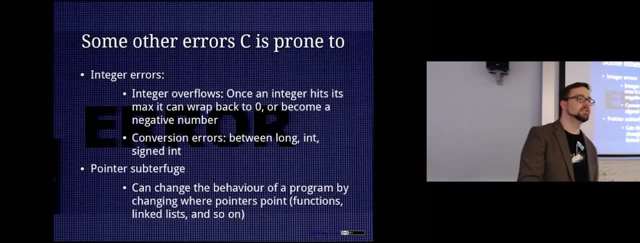 errors when you when you convert from like a long to an int or a signed int, and you can also have point assigns. So if you hit a number of a certain height, certain maximum number or minimum, if you're subterfuge, which is a whole category of programming mistakes where you basically 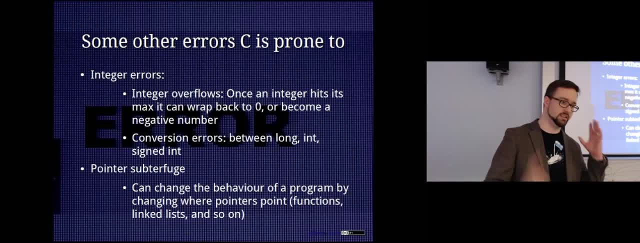 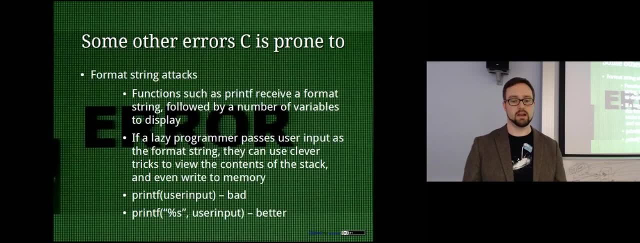 change where pointers are pointing at and you can have like functions and link lists and all sorts of things. Format string attacks is also a problem. So in this example here we've got printf user input. That's bad because actually printf should have a format string. So if you did printf 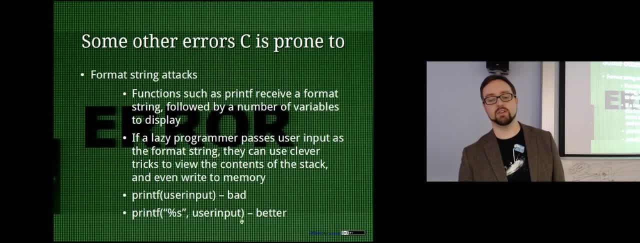